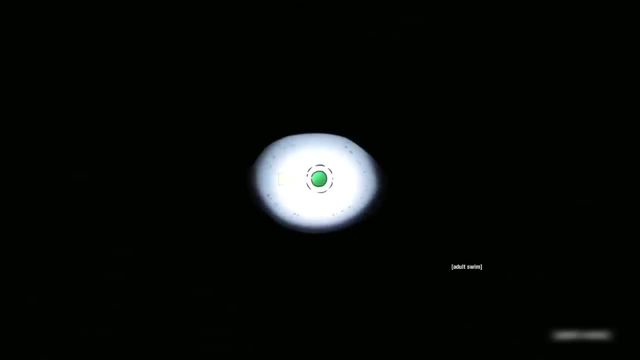 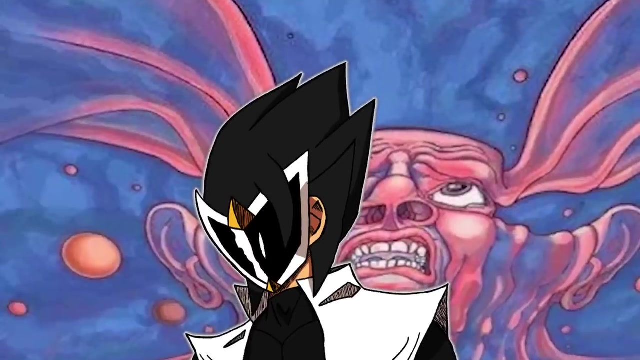 Crimson, but more or less the group that he leads, Passione, An Italian mafia group that basically kind of controls Italy secretly in part five, being led by Diovalo and King Crimson. Funny enough, the song itself references a lot of people in the court that more or less probably actually 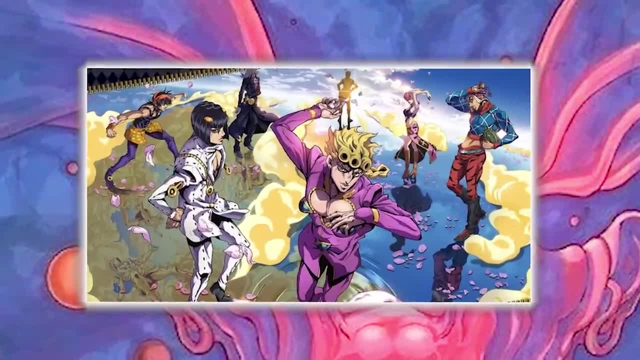 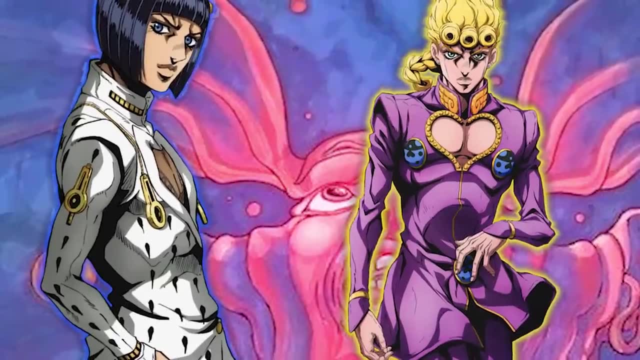 inspired a lot of the characters within Passione. Probably the two most I can probably figure out here would most likely be the jester being Risotto and one of the other few characters being maybe Bucciolati or Giorno maybe, But that is speculation at most. but you can see a lot of. 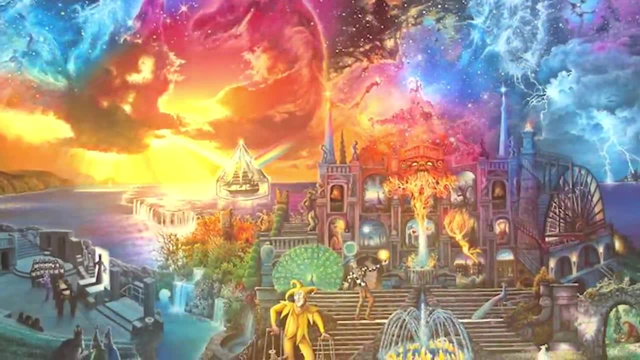 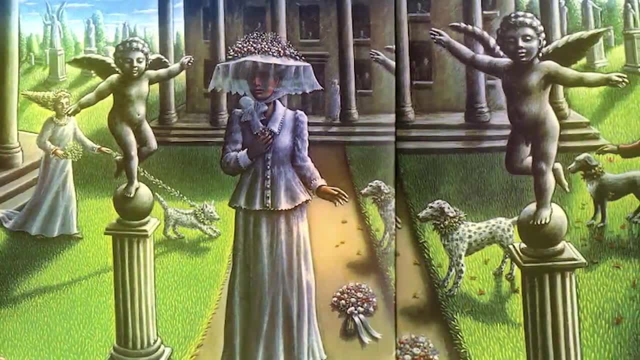 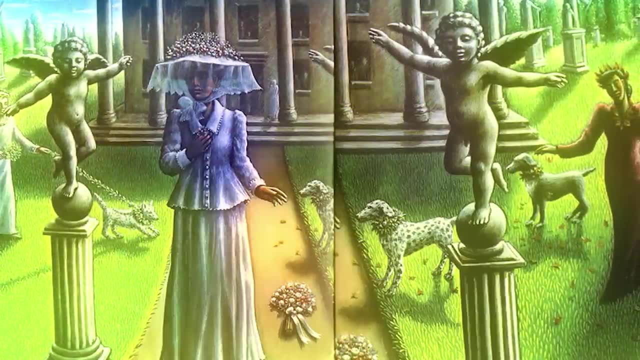 Next up being Epitaph, a song that probably inspires two things for Diovalo's character, One, of course, being the name of the substand, Epitaph- the ability to literally see ten seconds into the future, And second, most likely, Diovalo's overall character. Epitaph is a song about seeing. 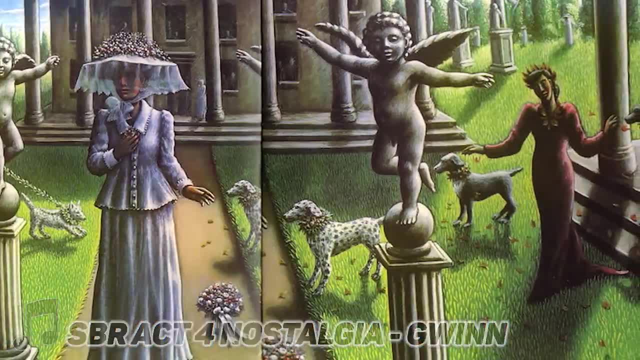 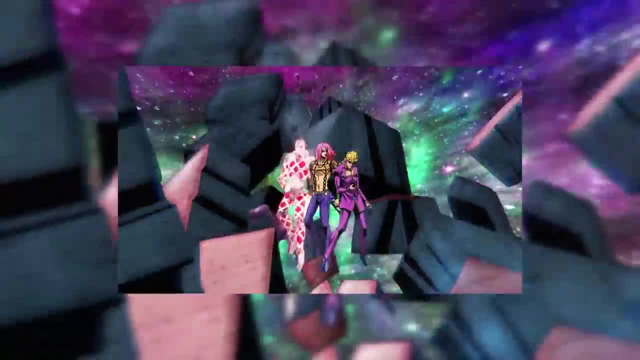 the nearby doom of the future coming forward and the yearning to want to change it. But instead of having a good result to the issue, more or less in Diovalo's case, it's probably making the situation worse, as he is now king of everything- bonus, you could also say. this song inspired the idea of the 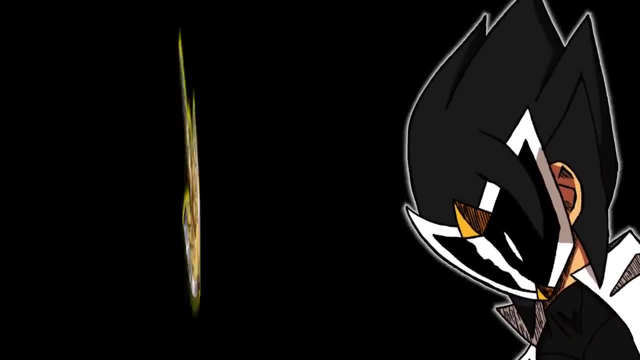 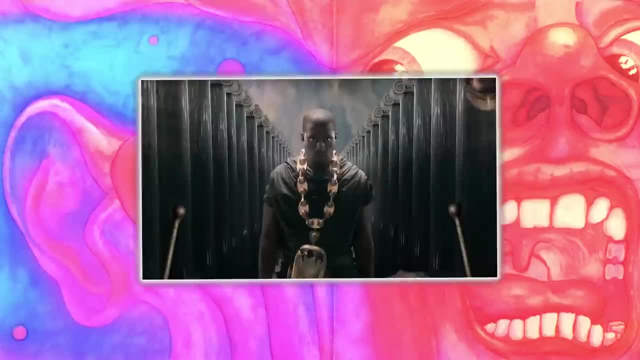 requiem arrow and stuff, but that one's for a completely different video, so i'm not really going to cover it here. next, 21st century schizoid man- probably one of the most well-known references here- thank you, kanye- is a literal song about a man with schizophrenia living in the 21st century. 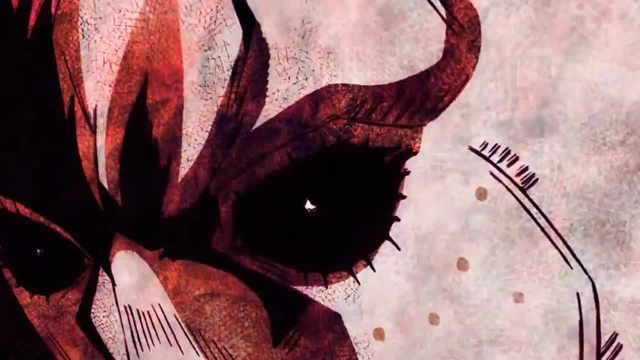 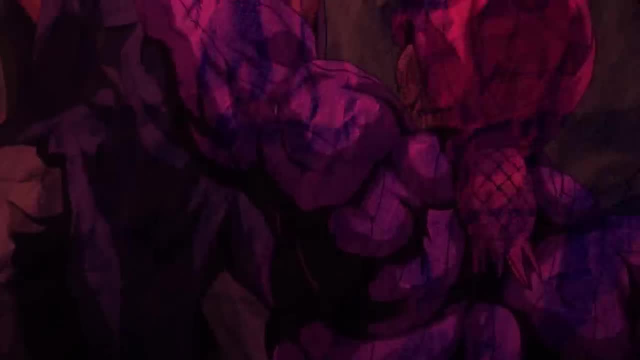 literally taking at face value by iraqi. dopio literally has schizophrenia. dio valo is literally a second personality. that is so bad that his literal body will transform into a completely different person. also, yes, i'm part of the crowd that thinks dopio is the main personality, as 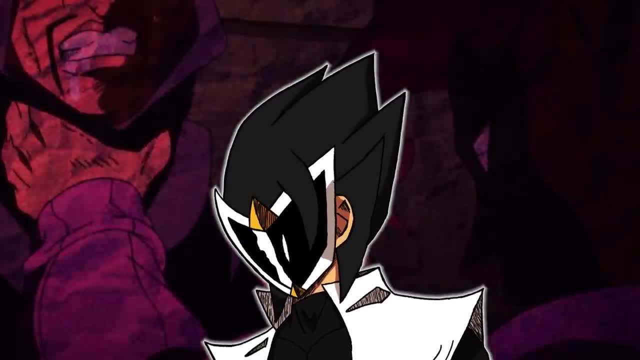 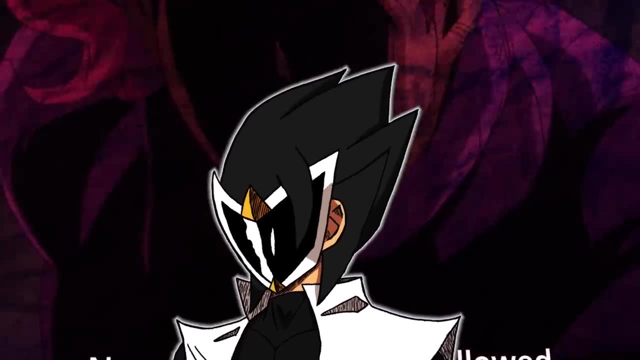 in literal schizophrenia cases, usually the second personality knows of its existence and knows about the main persons. the other main person doesn't actually know. the second one does. so in this case, accurately speaking, dopio is the main personality here, and that's all you need to really know before. 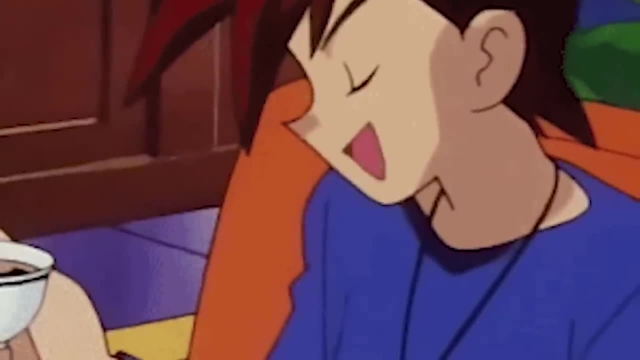 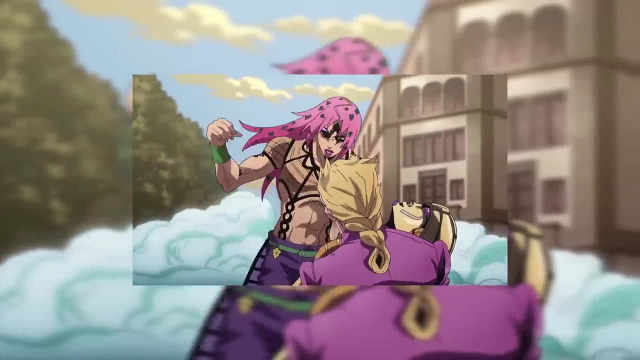 talking about king crimson, as more or less the entire basis of the idea of king crimson is this kind of thing of ruler or boss that's just kind of going crazy, that has this insane court and has these ideas of trying to overcome fate or trying to be fate itself and just overall just being a really creepy. 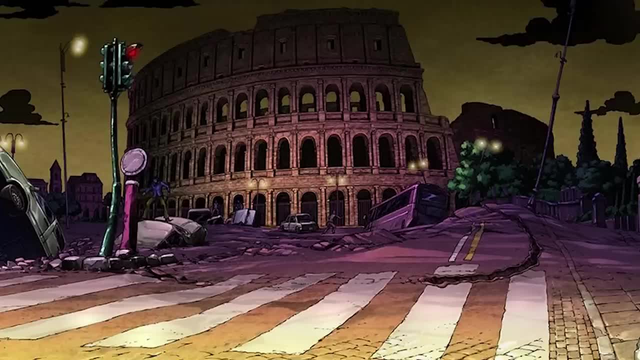 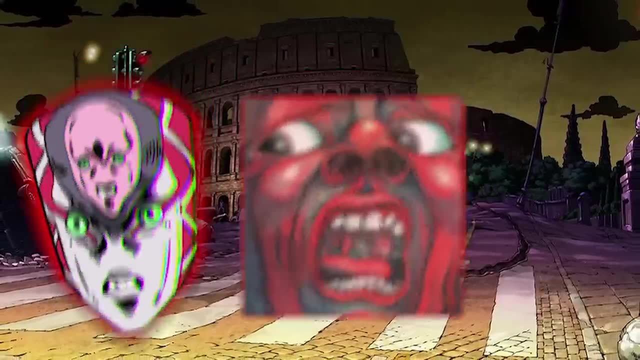 weird king kind of aesthetic that works incredibly well. but the other two references are kind of fun, of course the faces of the album cover literally inspired. you know, king crimson's weird ass looking face and most likely moon child is something that inspired trish's character. that one is kind of a. 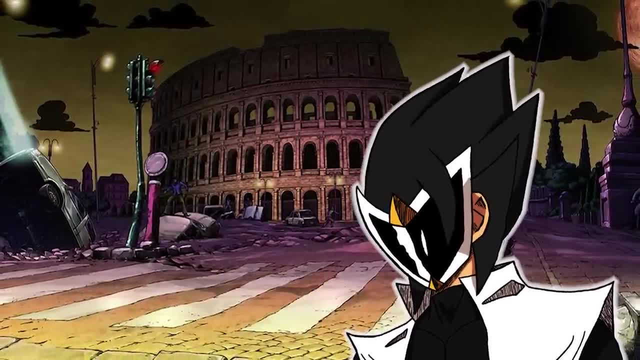 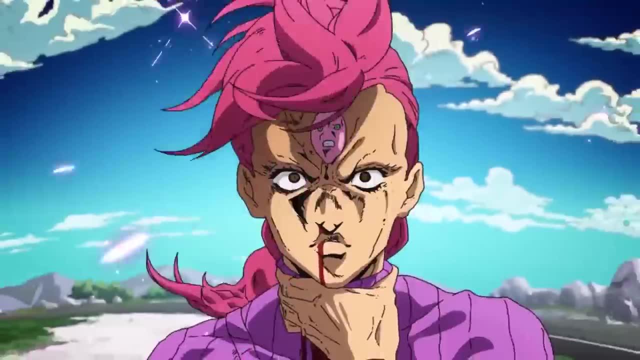 meta's original, and i don't see a lot of people talking about that one, but i think it's a good reference and i would like to point out a long reference sheet out of the way. let's finally talk about king crimson itself. so, off the bat, i'm going to explain this now. how does this ability work as? 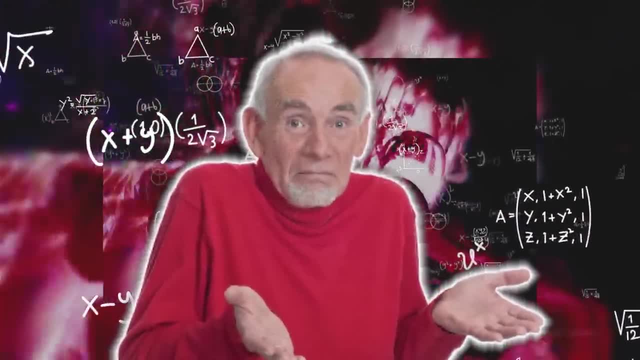 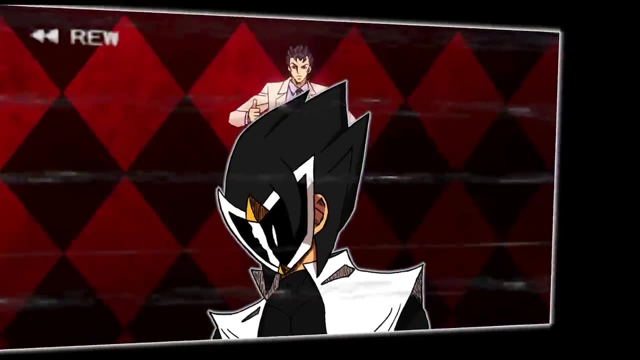 this is something a lot of people still find very confusing, so i'm going to break it down very, very simple and if you need to figure it out again, if you don't get it the first time, just replay this part, because after a while you should get it. i hope king crimson has two abilities, and i'm going to. 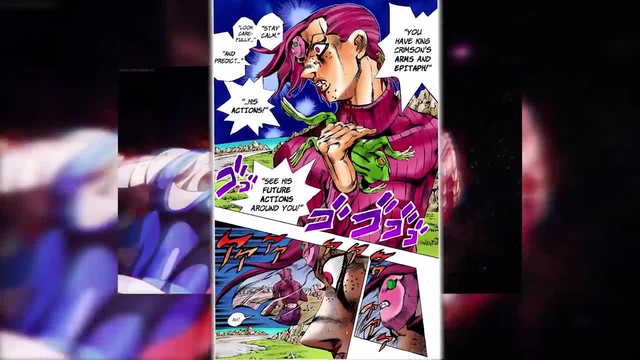 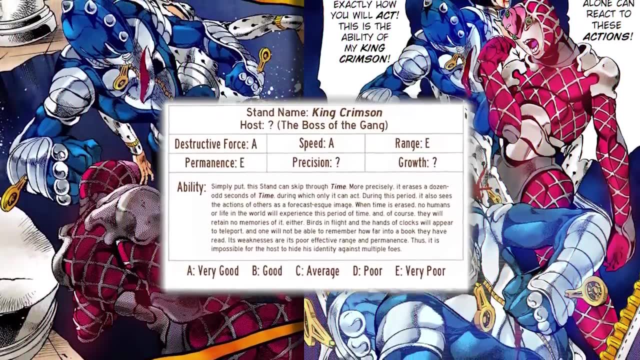 talk about his abilities, his time erasure and epitaph. epitaph has the ability to see 10 seconds into the future. that's it, nothing more, nothing less. time erasure has the ability to skip 10 seconds into the future, meaning that if there was any actions during the actual 10 seconds, only their. 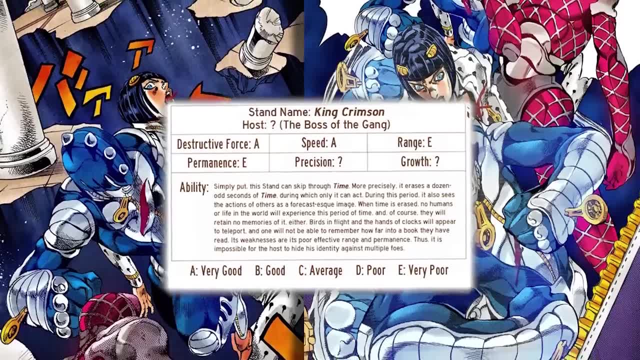 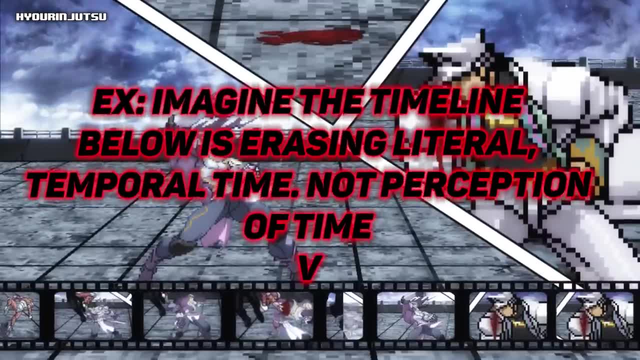 effects are left over, not their actions, as they have been skipped over, meaning that a lot of people have their perception of time erased. so more or less the idea that erasing something from the timeline is kind of wrong here is: it's more or less a lot of people's perception. 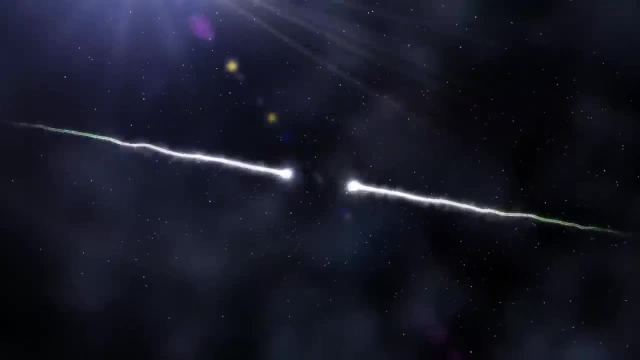 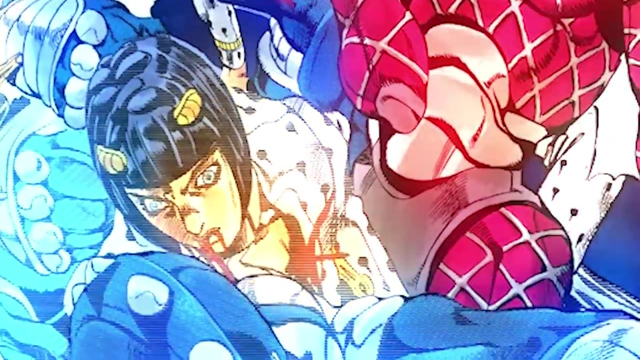 that is being erased, not the actual time stream, because that would lead to problems with the time space continuum. i'm not going to get into that, but more or less that's what kind of happens. it's your perception of time being erased in those 10 seconds. that's leaving a lot of effects behind. 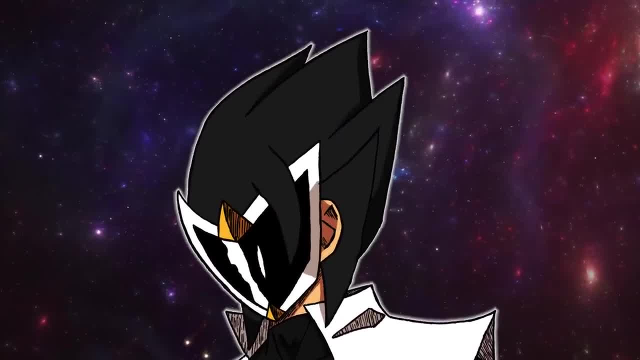 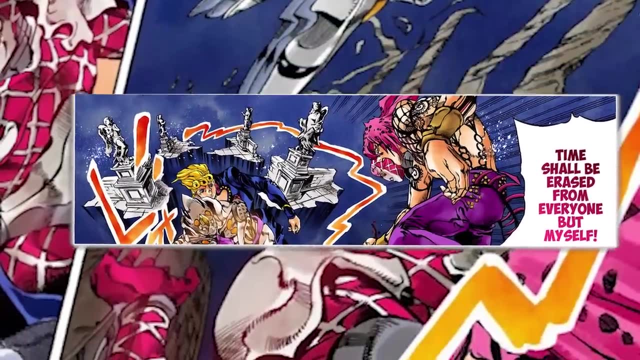 not the actions. mind you, it is still a time manipulation feat, as time is being skipped over, not erased. there are a few bonuses with this ability as well, as diovalo can move within this time skipping and cannot be hurt during time skipping. so pretty powerful ability by now i. 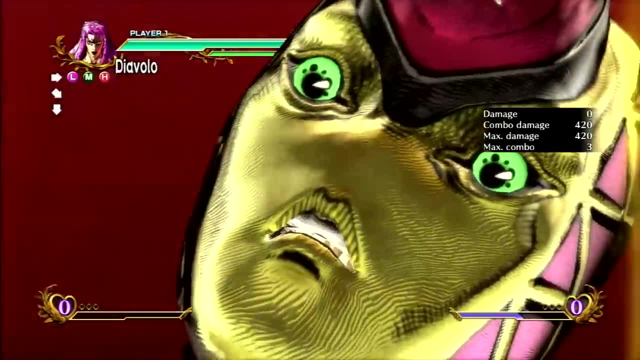 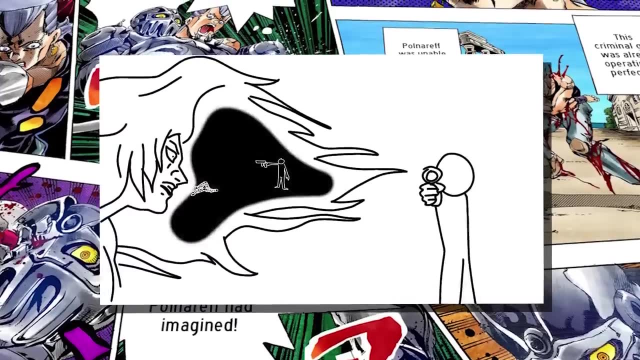 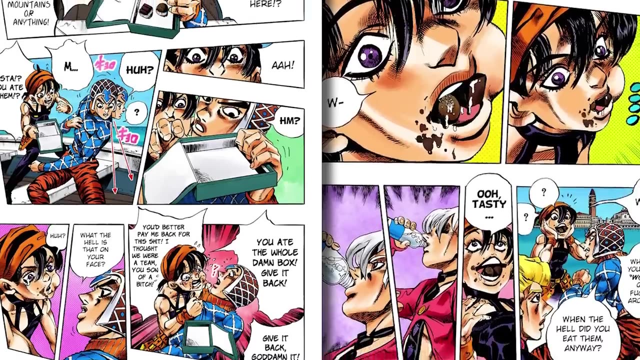 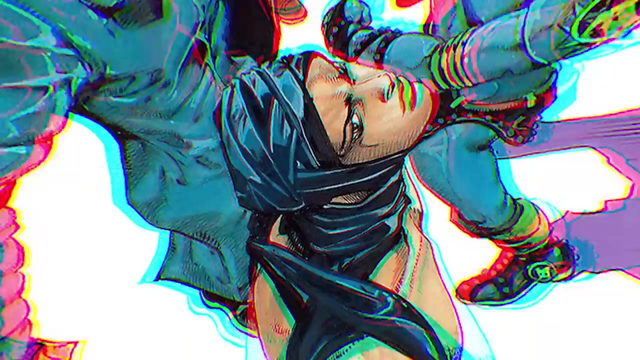 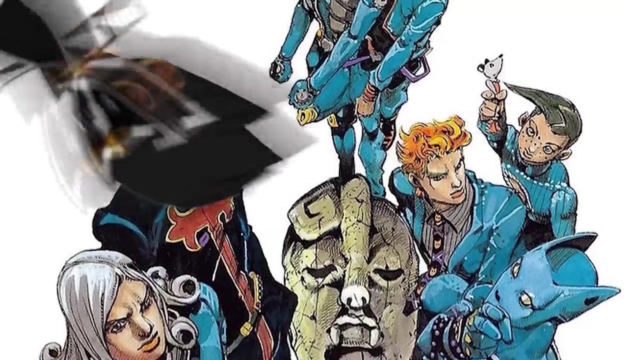 hope you're kind of enjoying this video. if you did, please leave a like and subscribe to my channel and i'll see you in the next one and i'll see you in the next video and i'll see you in the next video, and i'm meaning that very seriously. diovalo technically is like one really good ap feet. 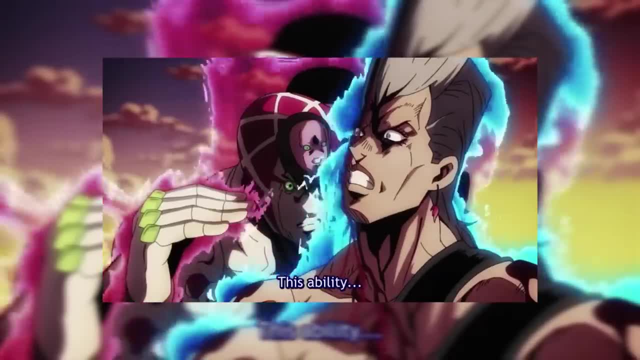 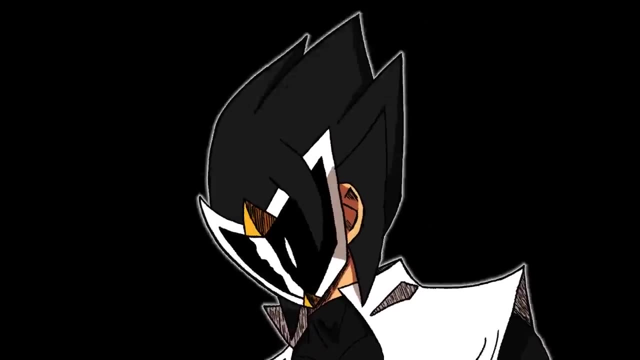 away from being one of the strongest to the point where he could probably defeat dio, jotaro and pucci with maiden heaven, not even joking there. and on the topic of scaling king crimson, let's talk about that in a time before part 5. john pierre polnareff would go to europe trying to. 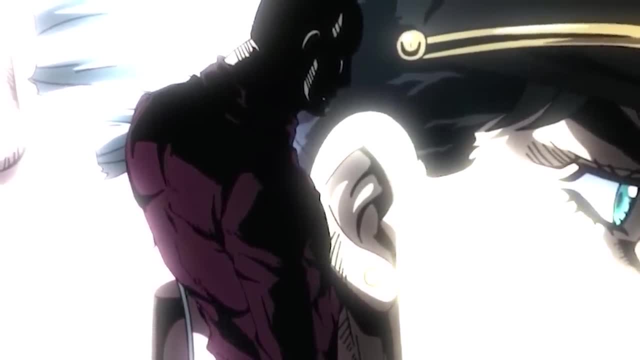 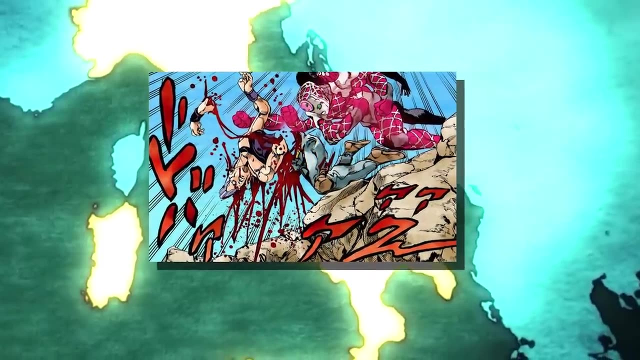 figure out why there was such a rampant drug problem, apparently diovalo. was this problem which would lead into an encounter between the two, which led to diovalo completely destroying polnareff? while i have stated this previously in other videos where this would just 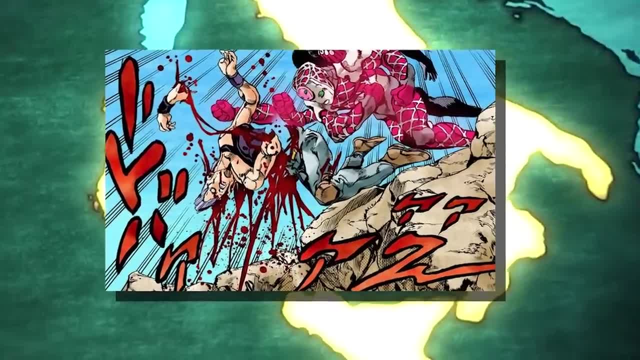 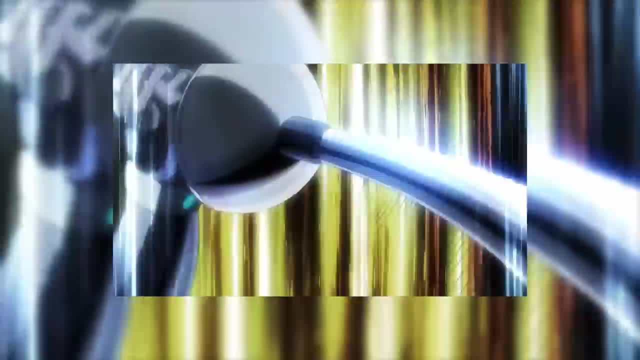 lead to a really crazy speed feat for diovalo. but there is something here that i haven't mentioned previously. we know that polnareff is an extremely experienced stand user. look at stardust crusaders, for an example. while, yes, polnareff is treated like a joke character for a majority of the time, 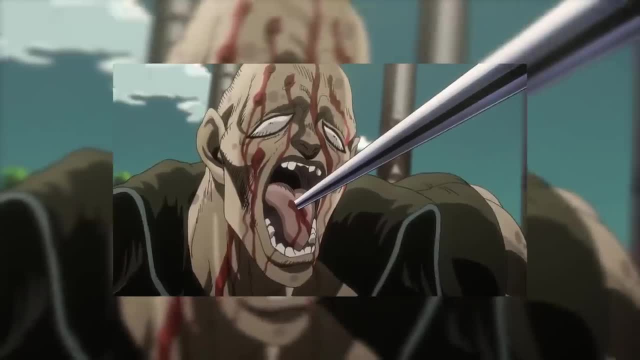 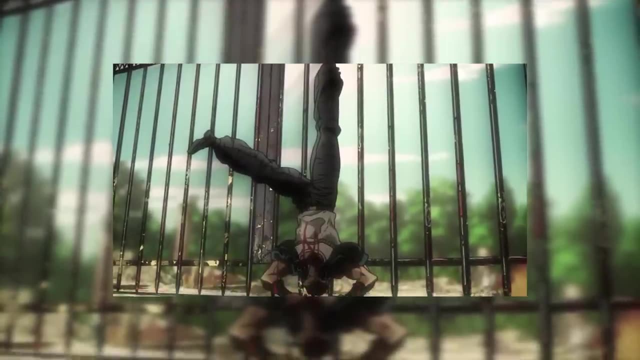 there is a lot of highlight moments with him that show that he is extremely powerful: the fight against hangman and vanilla- i should be great examples here to show you he outsmarts his opponents and even outlasts him in a way that i don't think he's going to be able to do in the 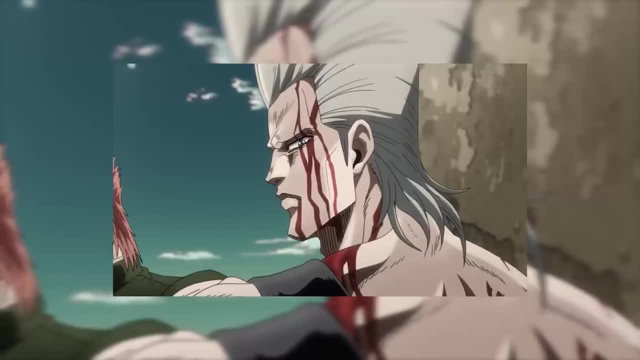 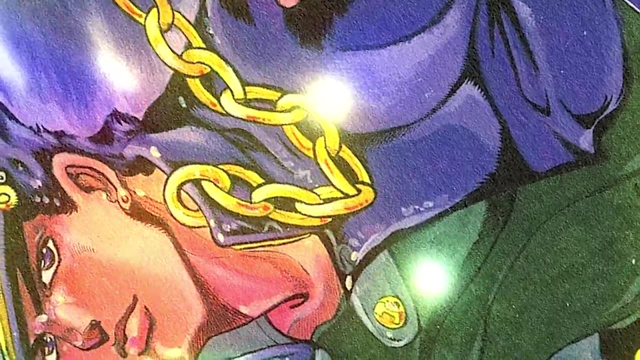 future, which is extremely consistent with polnareff. funny enough, because eventually he would be taken over by anubis and would fight jodorow, where even jodorow would consider polnareff an extreme threat. this is coming from the guy that has a stand that can reach massively faster than light speeds. 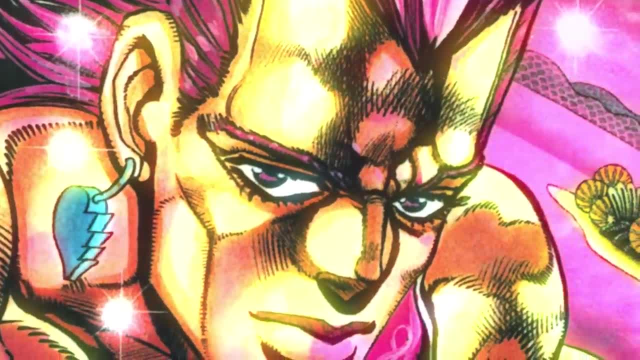 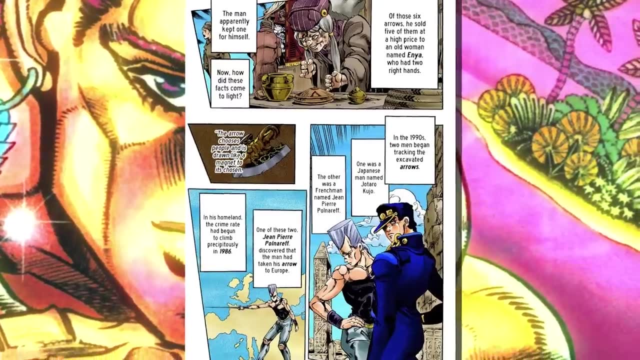 with city to mountain level. ap polnareff is no joke and is an extremely powerful character. it's even alluded to in part five that after part three, jodorow and polnareff would go on adventures together, meaning that polnareff probably got stronger and got more standing. 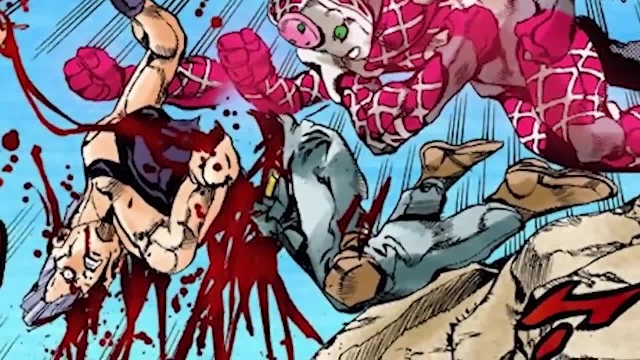 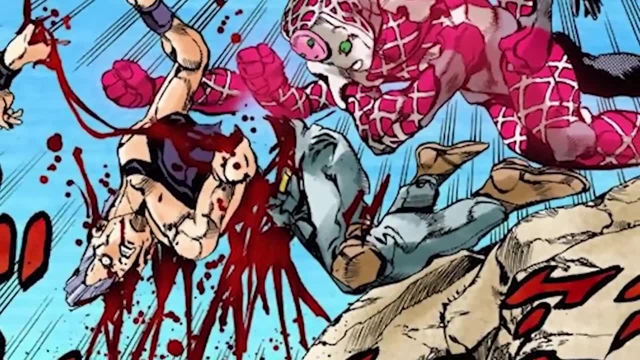 experience over this time span and then would get absolutely crushed and be disabled by king crimson and diavolo on a low ball, implying the fact that he at least has massively faster than light speeds, or you could say at least bare minimum, like this is the lowest. i would go faster than light. 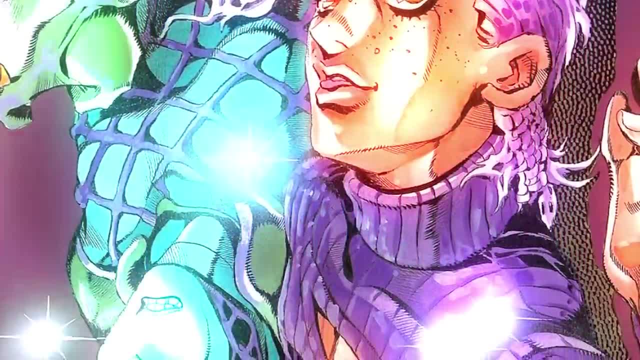 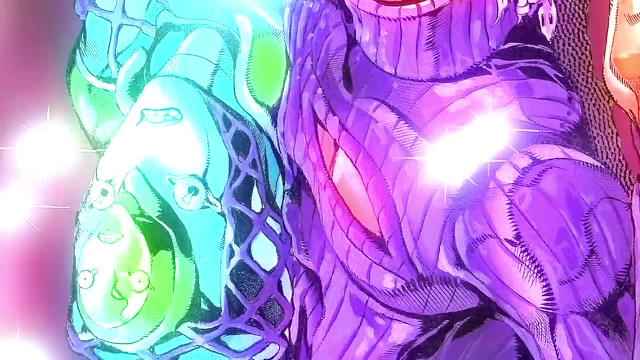 speeds and, like i said previously, he's like one good ap feet away from actually being an extremely powerful top tier in the universe. he is already, but like he's one away from being the top now, but i do think that he is not as powerful as the rest of his team in the end of the series. 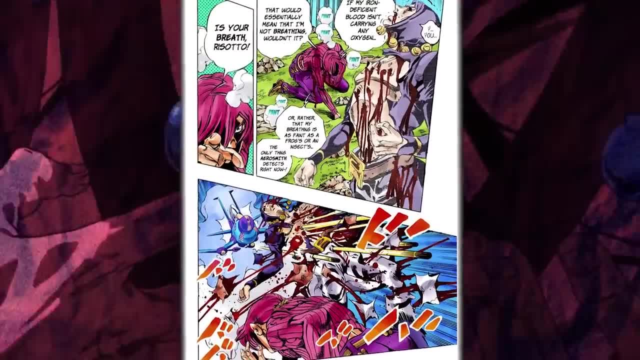 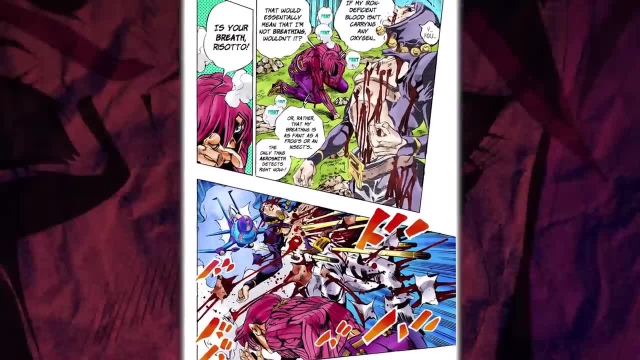 in terms of the amount of damage. he does make up for this lack of ap with other feats. the most wild one is being able to at least survive with a large amount of iron out of his system fighting risotto- there is only a certain amount of iron in the bloodstream, and the fact that dio valo. 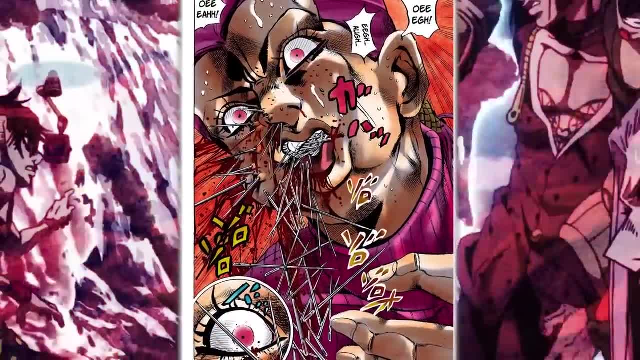 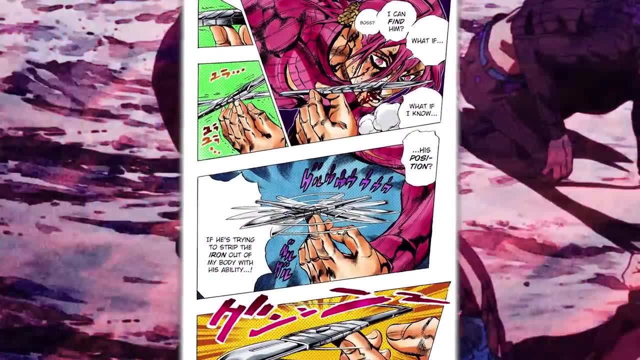 slash doppio here had so much he was able to make a large amount of iron weapons and survive being attacked with them by risotto, making this a really good durability feat. and shortly after this, he would use his intelligence and his nearby surroundings- Rizzotto, making that a really good intelligence feat for him, which is really consistent with 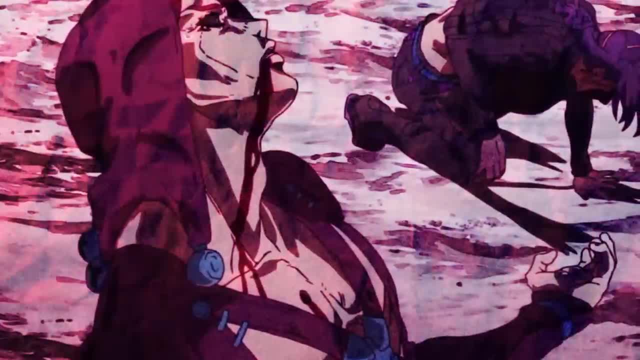 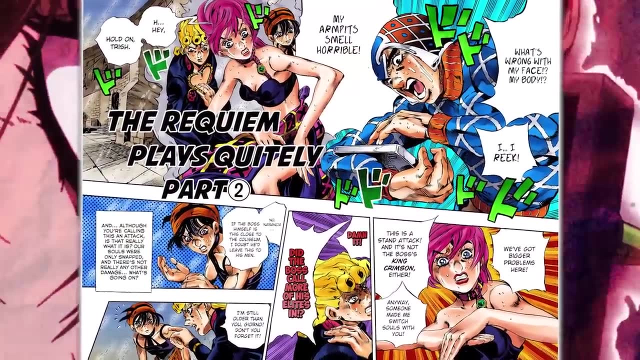 his character, As shortly after this in the Requiem Quietly Plays, he would use the confusion of Silver Chariot Requiem to get closer to the Requiem Arrow. While he did end up losing the Arrow, the fact that he was able to pull off confusing the group for so long is still really. 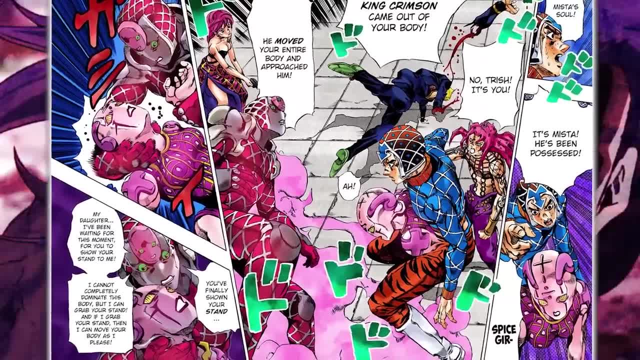 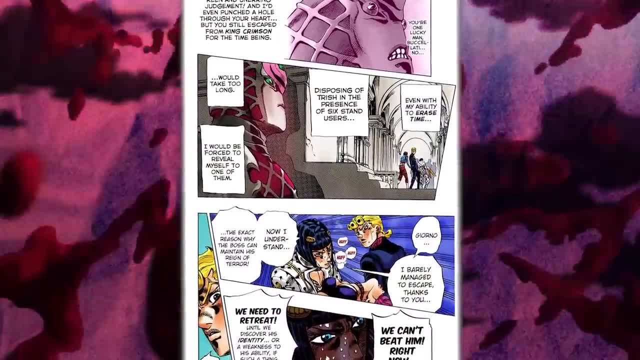 good on his part, slowly biding his time, trying to get closer to the Arrow. The only thing holding him back was, well, Silver Chariot Requiem. As in an earlier encounter with Bucciarati, literally in his introduction, he probably could have taken out the entire team. The only thing. 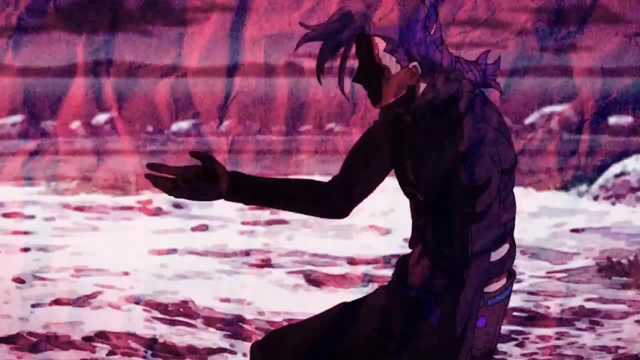 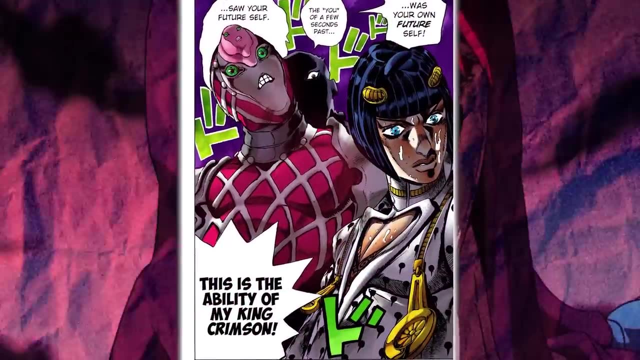 holding him back was he didn't want anybody to see his face. If previous intelligence feats and speed feats are to be taken in mind here he probably could have done it. It's not him just hyping himself up thinking that he's the greatest in the world. He has the stats, the time skip. 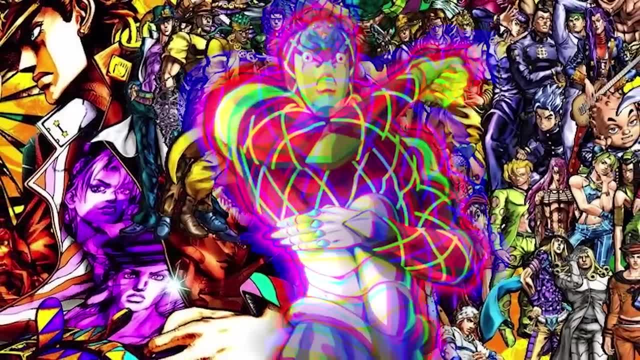 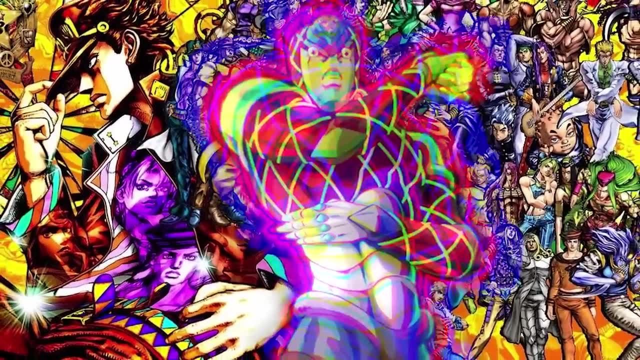 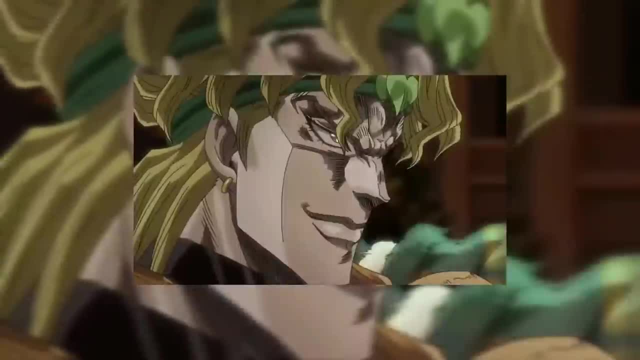 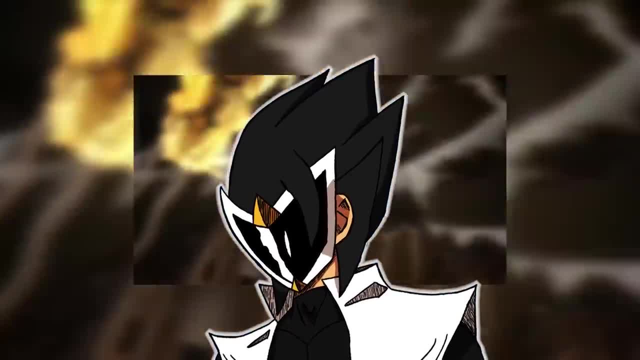 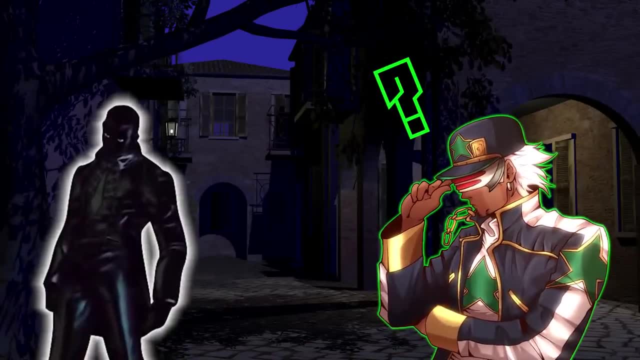 Meaning that the line of error or losing is extremely small, So small, in fact, that you can probably count them all on your hands. So if you ever were to encounter Diovalo in a real life situation, or meeting him for whatever reason, you're probably gonna die. Hands down. 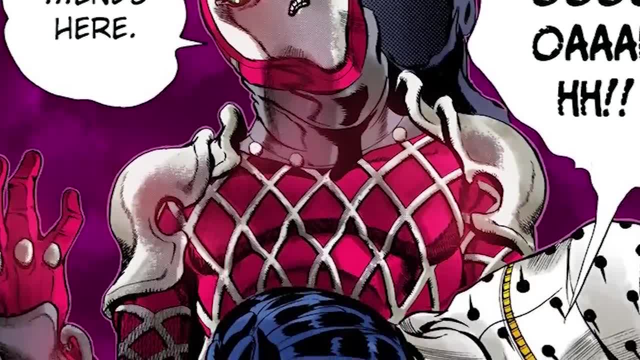 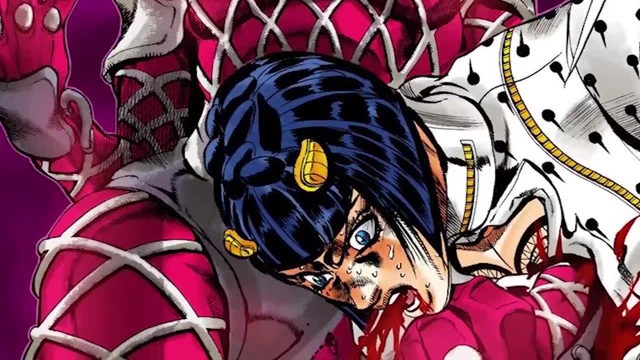 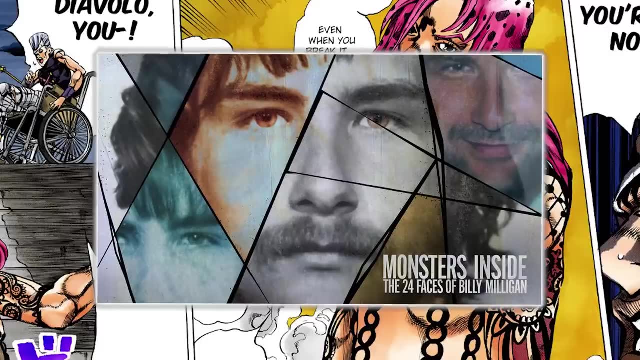 Even a regular stand user probably doesn't even stand a chance against this guy. Time skip and precog are just that broken And it possibly gets even worse if you know, the more deeper Jojo stand lore. You see, Diovalo is technically based on Billy McGillen, Or at least his condition. He is a man. 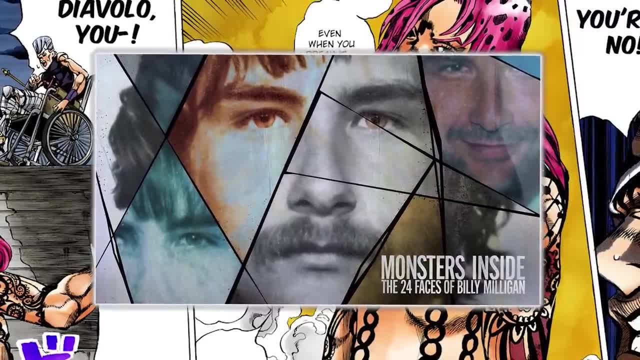 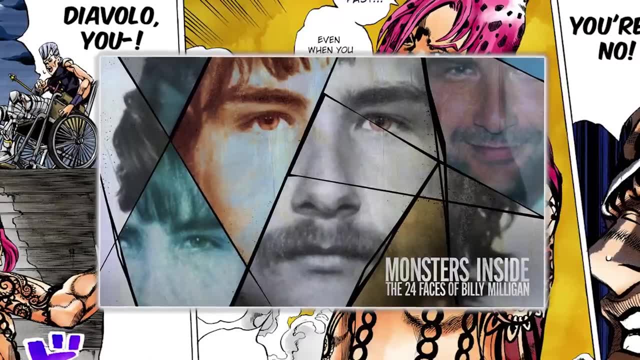 with multiple personalities And, to cut a story short, at one point all of his multiple personalities merge into one perfect personality. I guess is the best way I can quote it- making this kind of super character that was radically different from the main one for some time with. 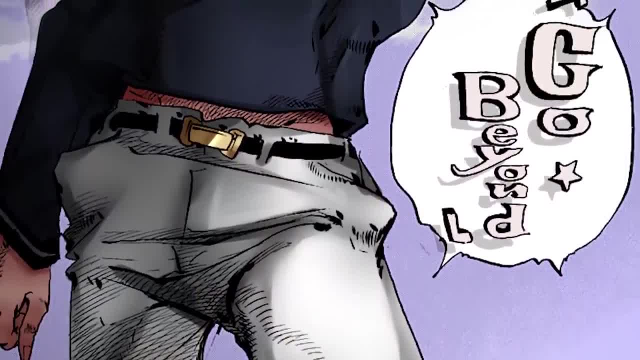 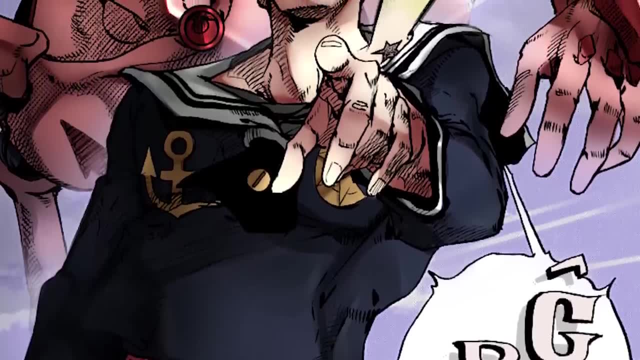 Billy, And thanks to Part 8 to Join. we know that if a person were to go through a crazy resolved change or a crazy life circumstance thing happening with them, a stand evolution or a stand change can occur, where maybe a new ability forms, Of course, being an example here being 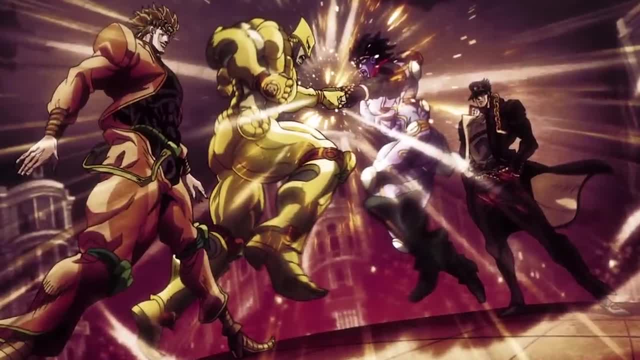 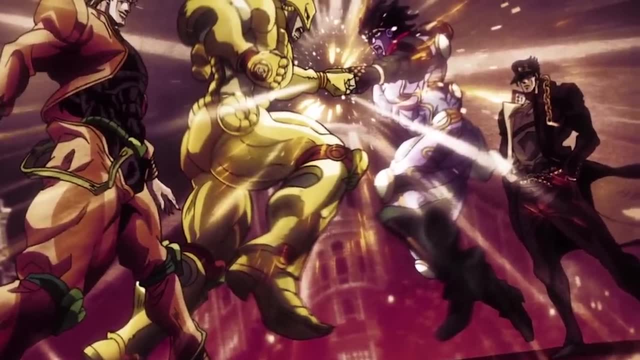 Soft and Wet, Go Beyond And even previous to Part 8, that we know that act stands or maybe even a change in power. that being an example here would be Jotaro Kuja, with Time Stop, being in an extremely pressured situation, losing his loved ones and his friend group. a stand evolution or a stand change. 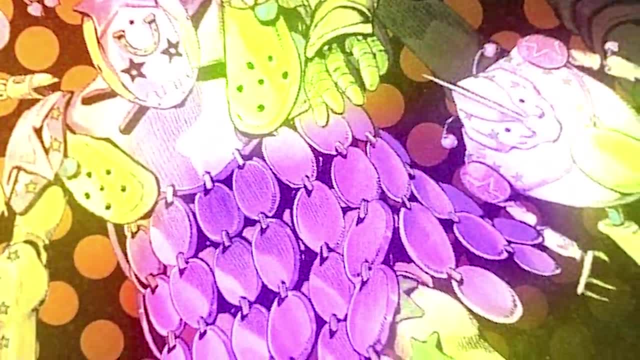 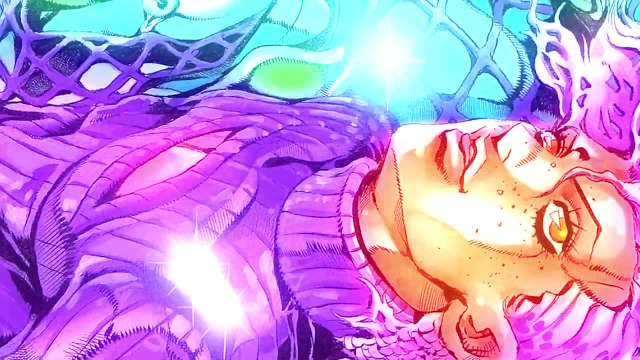 in power can occur. An example of the acts would be Echoes, Act 1-3, or Tusk, Act 1-4.. So in this example, if Dopia were to become self aware of Dio Vallo and maybe some type of multiple personality fusion were to occur, this could. 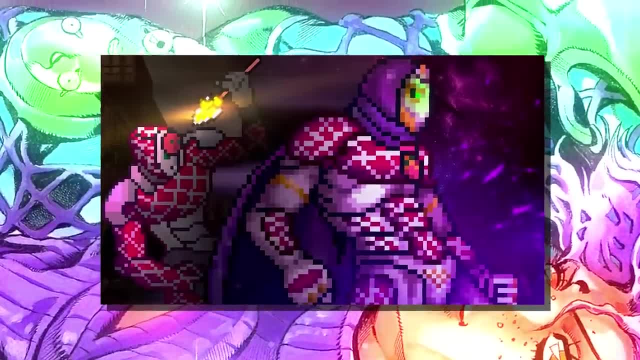 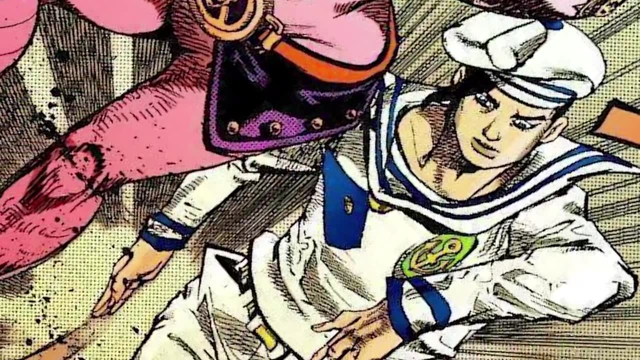 possibly lead into a completely different or even a stronger version of King Crimson. Note. I would like to add upon all of this: this is just fan speculation on how certain things work in this universe. Even if this doesn't occur, King Crimson by himself is still extremely powerful. 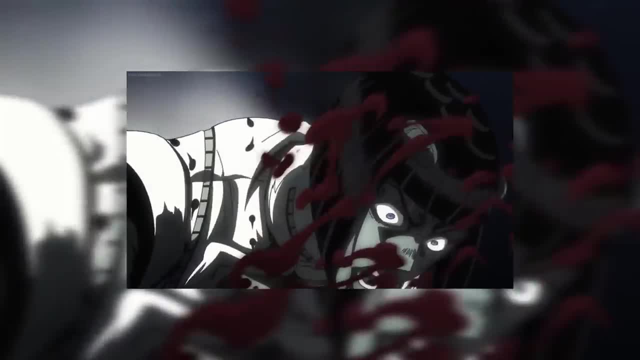 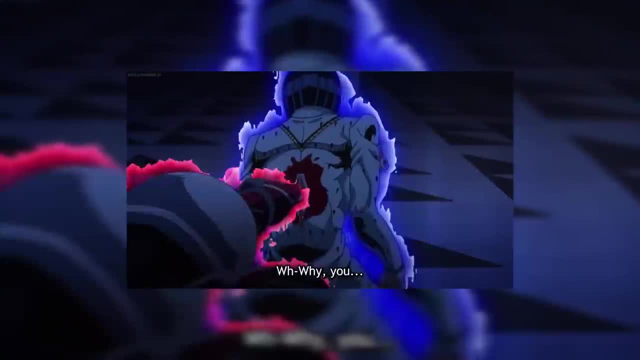 like I've said previously, I would probably even say he's probably one of the most powerful and intelligent villains in the series And, paired up with a stand that can have the ability to see the incoming fate and able to skip over it, is extremely good and powerful.